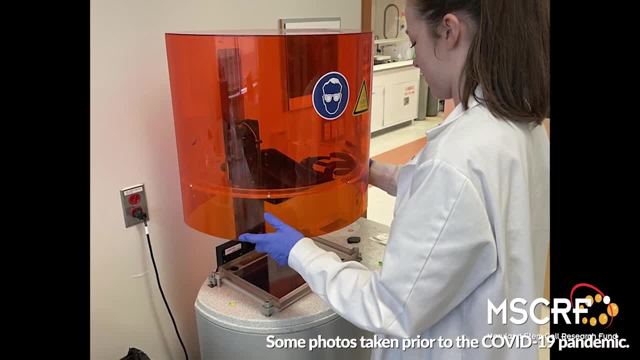 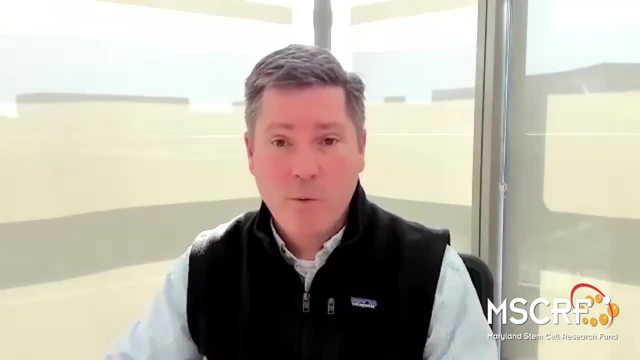 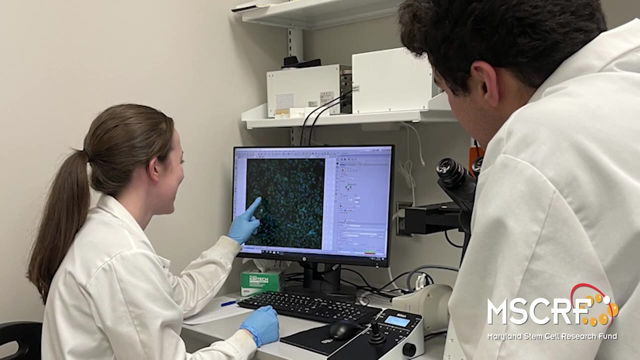 tissues within the laboratory as replacement or engineered tissues that can be put into a person after the tissue loss. So we look at building them in the laboratory as well as building culture systems that help grow these tissues in the laboratory. We've done this work for a number of years and key technologies that we've developed 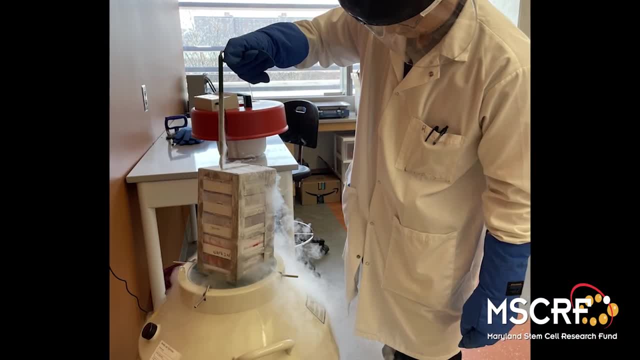 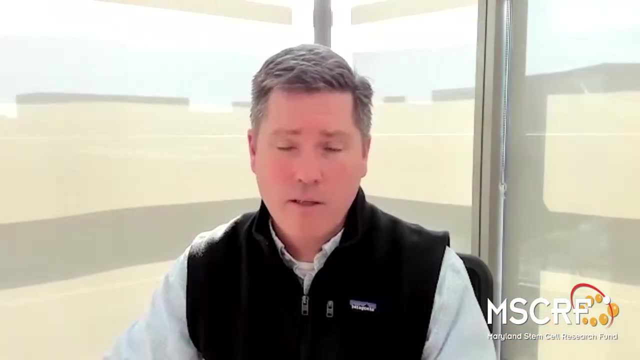 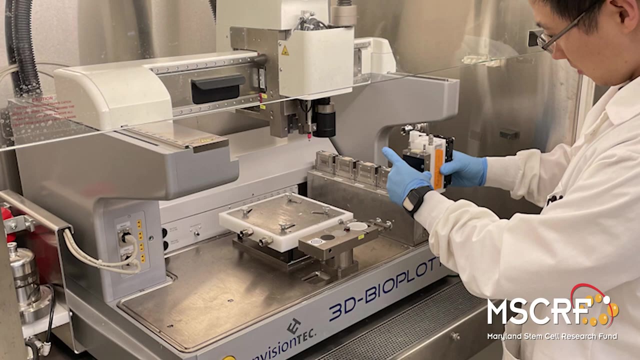 in the lab include 3D printing approaches for fabrication of materials and stem cell based construct, as well as bioreactor technologies for growing and culturing engineered tissues. The emerging areas of printing- 3D printing and bioprinting- really have a lot of power. 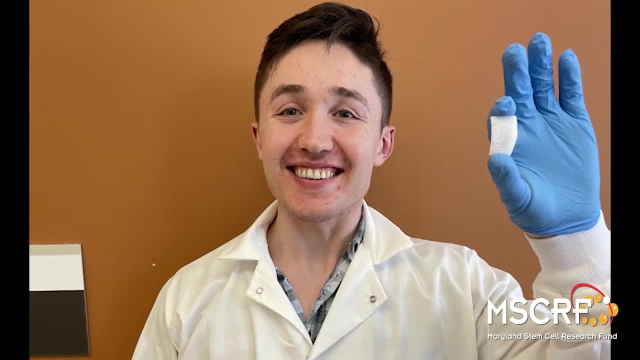 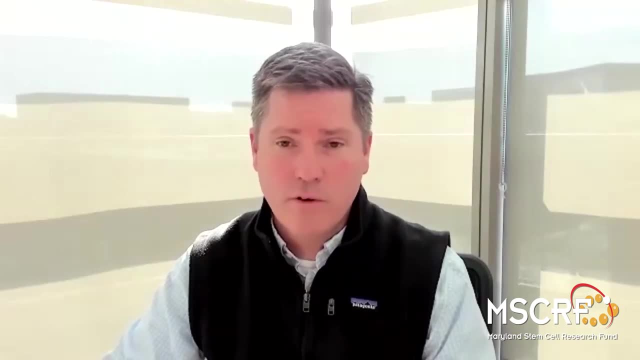 to try to replicate the complexity that we see in native tissue. We've been very fortunate over a number of years to receive support from the Maryland Stem Cell Research Fund. I believe we were the first lab on the College Park campus To receive an MSCRF research grant. I think it was way back in 2007,, among the first class. 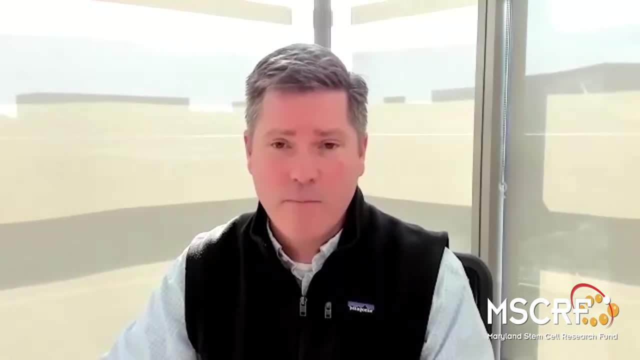 of folks that received funding from the state. We've been able to use this funding to grow our lab and our lab's expertise in the areas of tissue engineering or regenerative medicine. Particularly, we focused on areas including craniofacial regeneration and in collaboration. 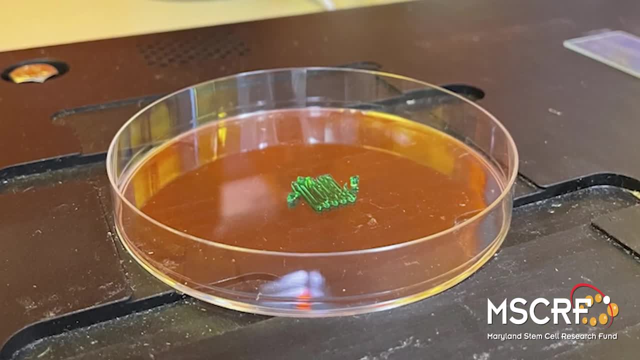 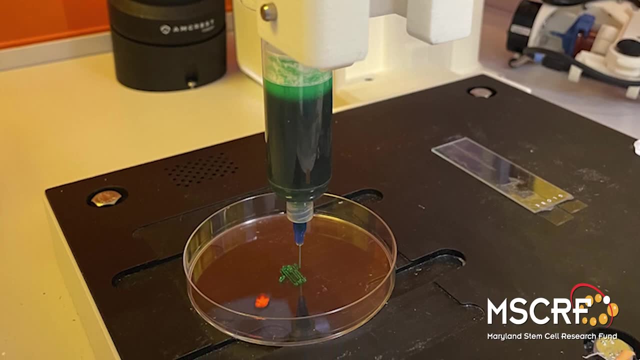 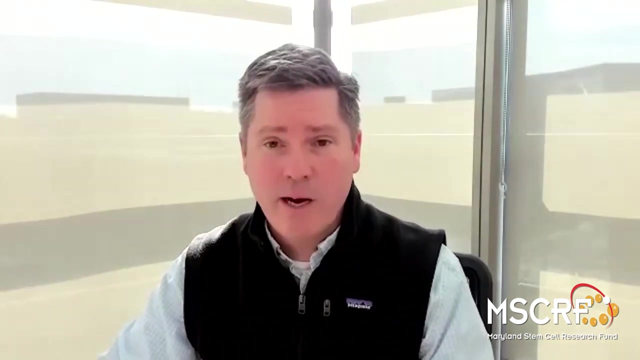 with folks in the Department of Oral and Maxillofacial Surgery in the School of Medicine. In addition, we've looked at areas including engineering bone marrow or co-cultures between mesenchymal stem cells and hematopoietic stem cells, and we've done this in collaboration. 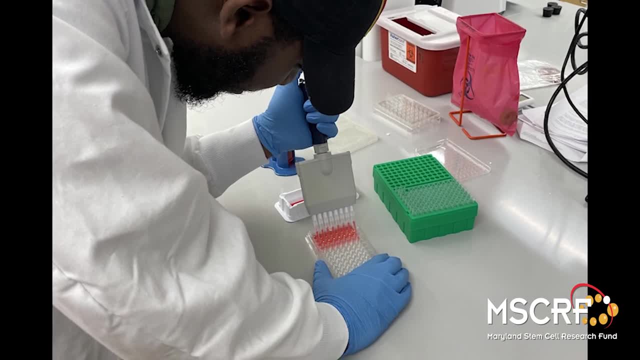 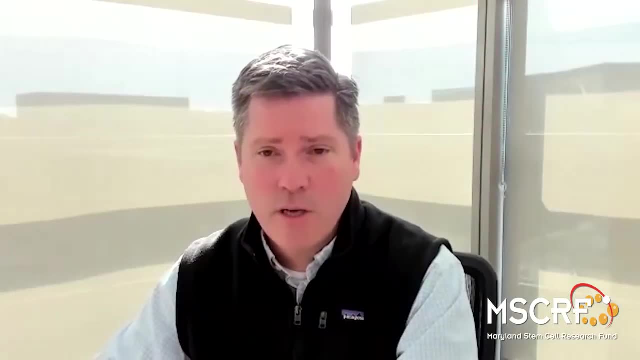 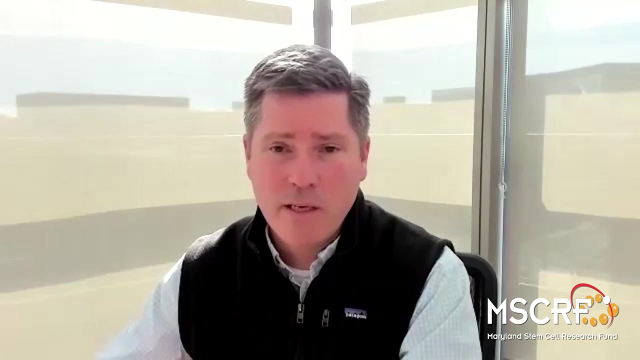 with folks at the School of Medicine as well. I think without the work that our lab has accomplished, as well as our colleagues throughout the country, We're really limiting the ability to think about the replacement and regeneration of lost tissues, For instance, in cancers involving the bone. this can impact pediatric patient populations.